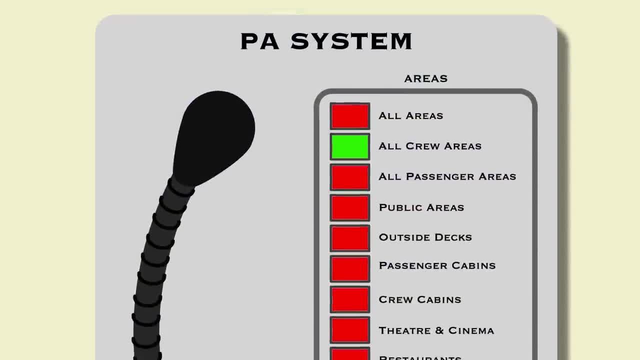 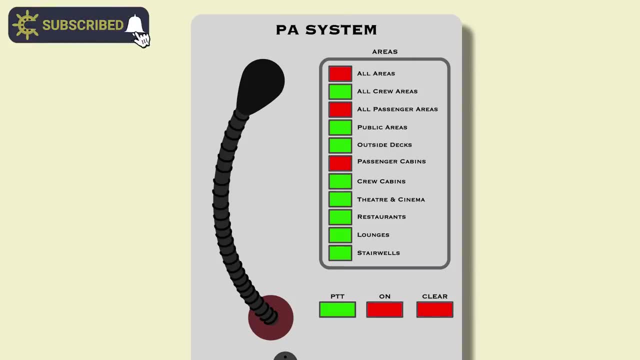 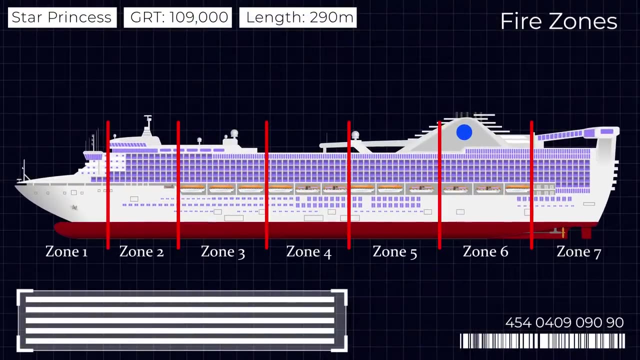 the port side of the ship's superstructure. The officer on watch activated the ship's emergency response by putting out a broadcast over the PA Assessment party. proceed to Zone 2, deck 11.. Ships are divided into a series of fire zones, separated by A-class divisions. 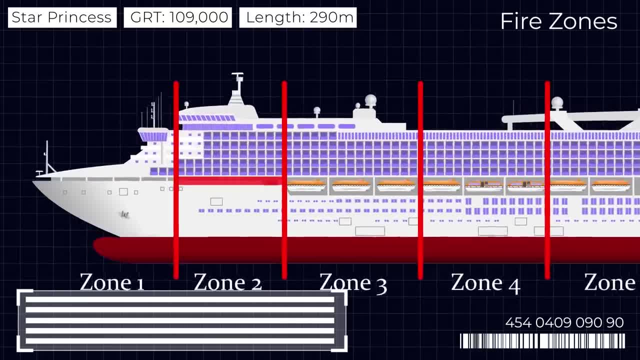 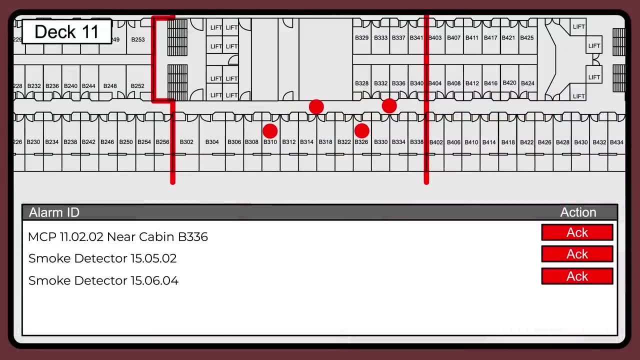 Star Princess had seven such divisions. so Zone 2, deck 11, told the assessment party to head to the forward end of the ship B deck. On the ship's fire control panel alarms continue to activate, with a series of smoke and heat detectors and a flow alarm from the high fog. 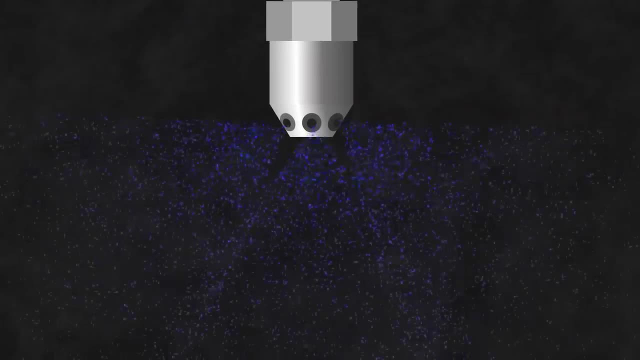 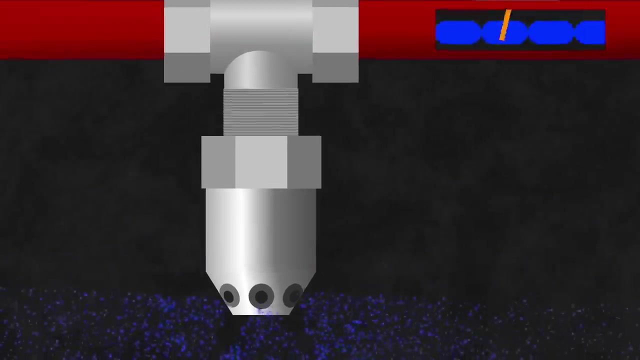 High fog is a pressurised fire protection system that produces a fine mist. when a glass-filled vial is broken by a rapid change in heat, such as you'd expect in a fire, The flow of water to the mist head activates the flow alarm indicating the system has 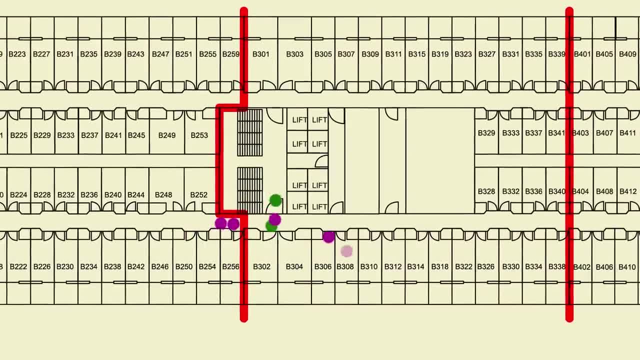 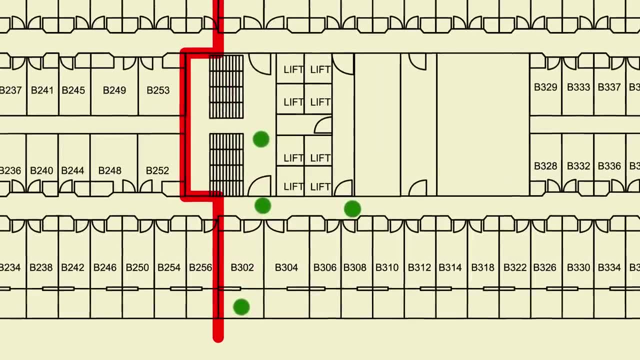 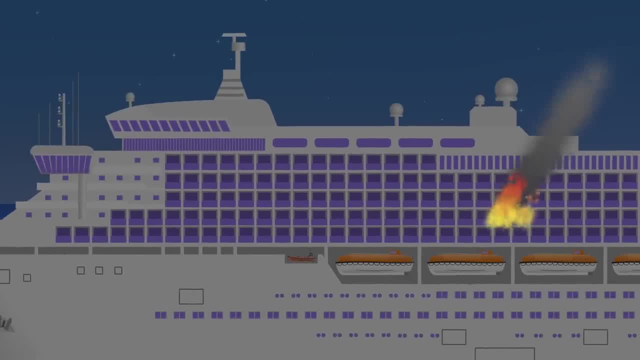 started On deck. the assessment party were met by passengers already leaving their cabins. Immediately, they requested crew alert, which would summon all crew to their emergency stations. Back on the bridge, the captain and deputy captain had arrived. Having been woken up by the original broadcast, they could see that the fire was on the balconies. 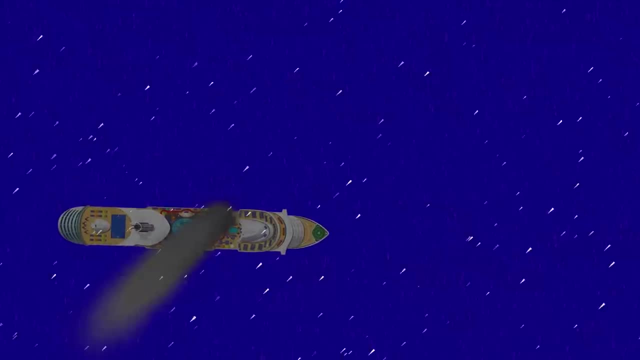 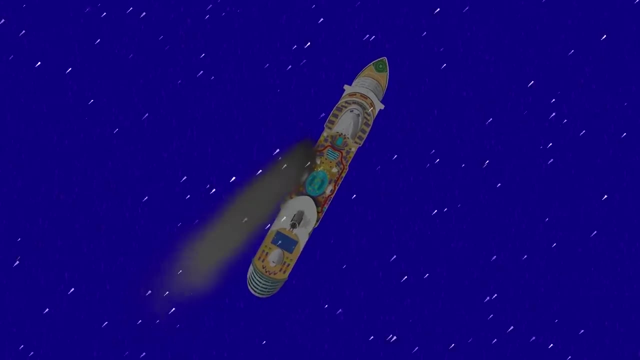 spreading aft, driven by the wind over the deck, The captain ordered the ship's speed to be reduced and he altered course to place the wind on the starboard bow. to try and help the smoke drift away from the ship, The deputy captain went to the ship's emergency response centre just behind the bridge, where 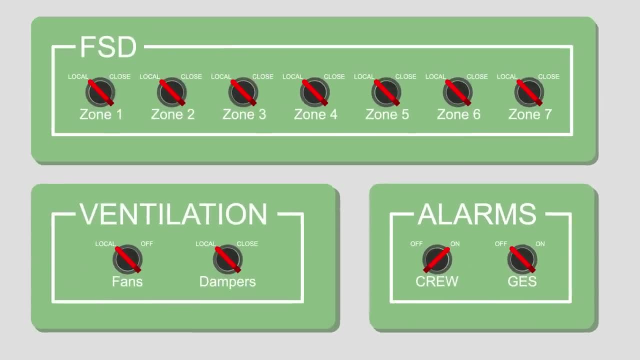 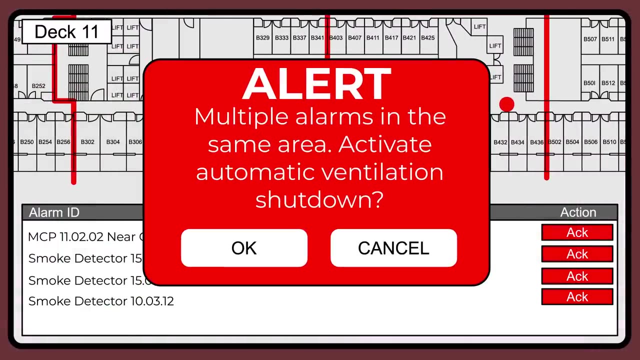 he activated crew alert, started remotely closing the fire doors across zones one, two and three and shut down ventilation using the master switches. Automatic shutdowns had already kicked in thanks to the fire system, but it's best to make sure with those master shutdowns. 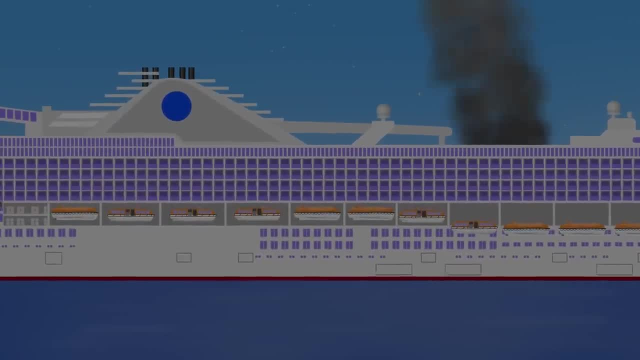 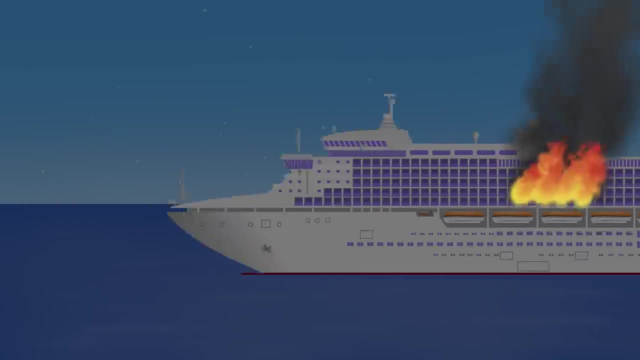 With the crew alert sounding, all crew were sent to their emergency stations to prepare to receive passengers. Lifeboats on the starboard side were swung out and readied, but the ones on the port site couldn't be prepped as they were so close to the flames. 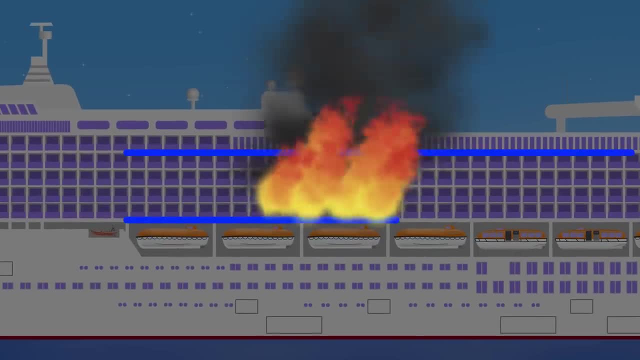 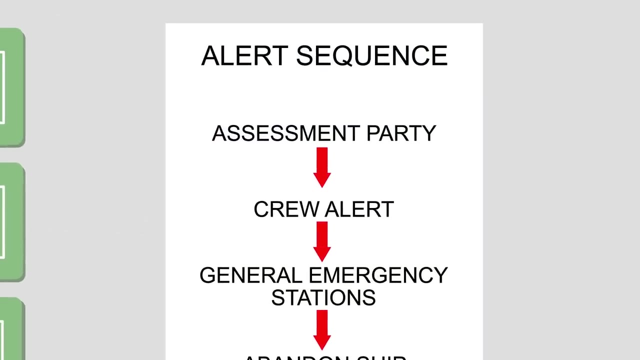 Boundary cooling was soon established around the fire, initially on deck 14 above and on deck 7 below, to protect the lifeboats. With no prospect of a quick resolution, though, the ship quickly moved from crew alert to full general emergency stations, summoning all passengers to their muster stations. 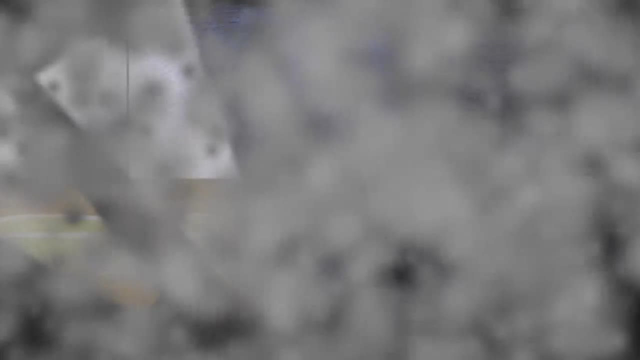 At the scene of the fire, teams in full breathing apparatus were deployed to search cabins for anyone that might be trapped. Although the high fog system was proving incredibly dangerous, the crew had to be prepared to deal with it. While it was incredibly effective at keeping the fire out, it couldn't do anything to 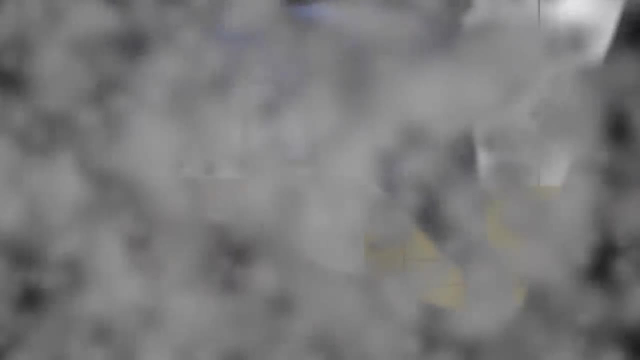 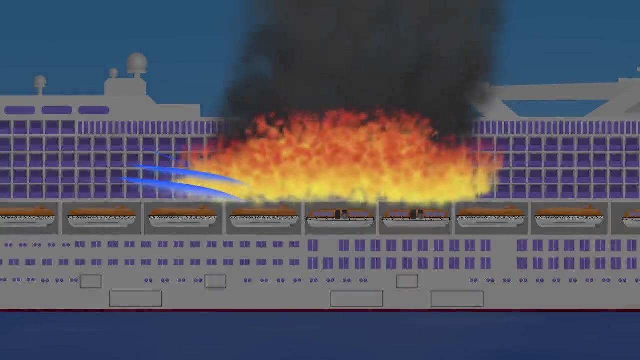 stop the smoke. Firefighters had to crawl through feeling their way around because the visibility was so poor. As the high fog contained the fire to the balconies, the main effort to extinguish the blaze was focused there. Hose parties with smoke masks were deployed to adjacent balconies to dump as much water. 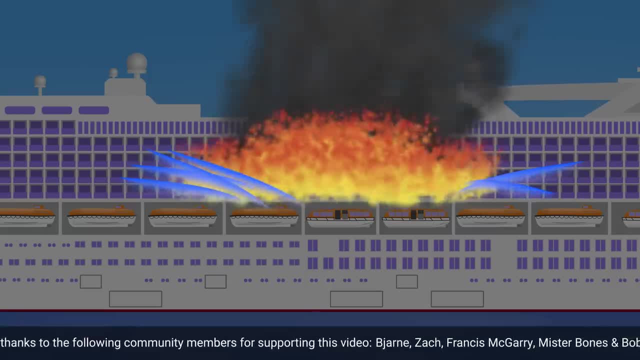 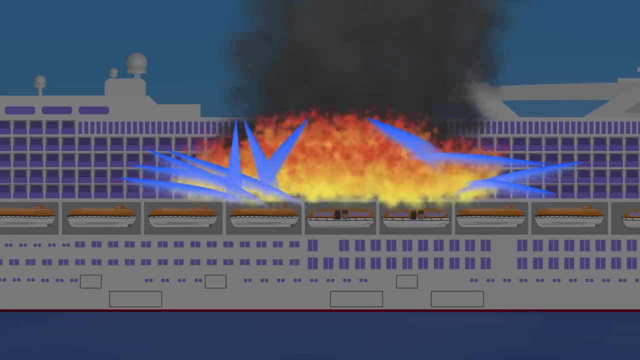 as possible on the seat of the flames. At 0340, within 30 minutes of the first manual call point activation, at least 7 hoses were fighting the fire in zones 3 and 4, with another 5 fighting from deck 15 above. 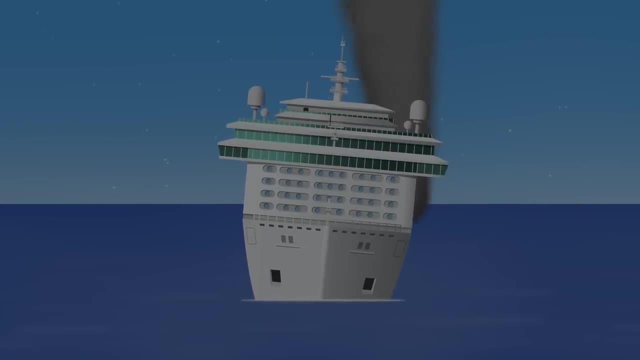 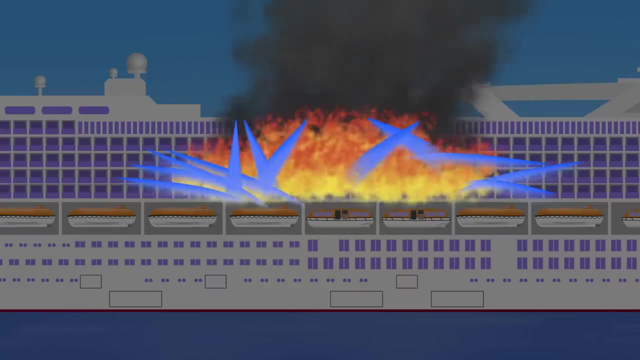 They were using hundreds of tonnes of water. so to avoid capsizing the ship, they applied a port list so that it would all safely run away. By around 4am the fire began to reduce in size and by 436 the captain was making an. 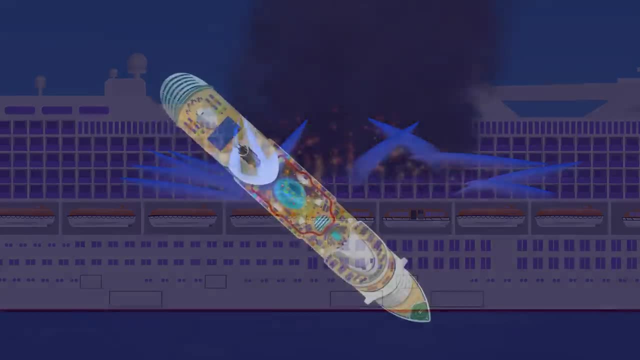 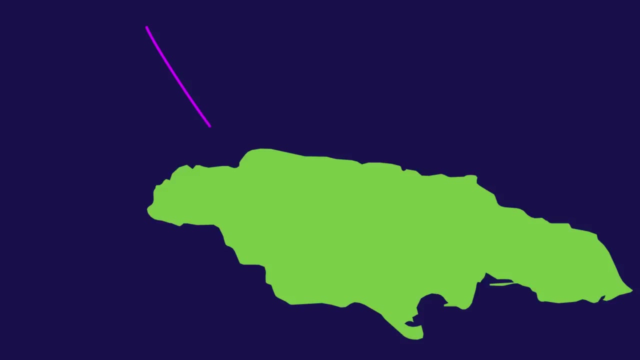 announcement telling everyone that it had been safely extinguished. The crew spent the next hour or two searching the affected area, after which the captain decided it was safe to resume passage to Montego Bay. The captain then decided to leave the area and return to Montego Bay. 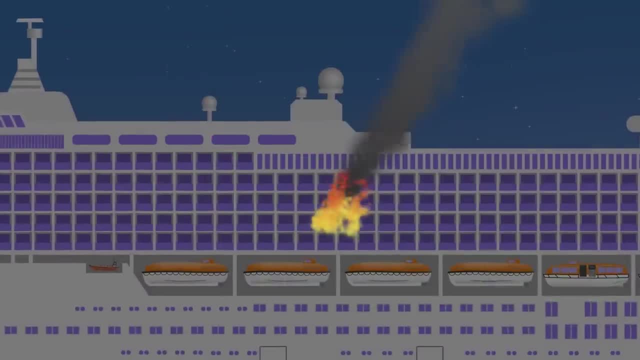 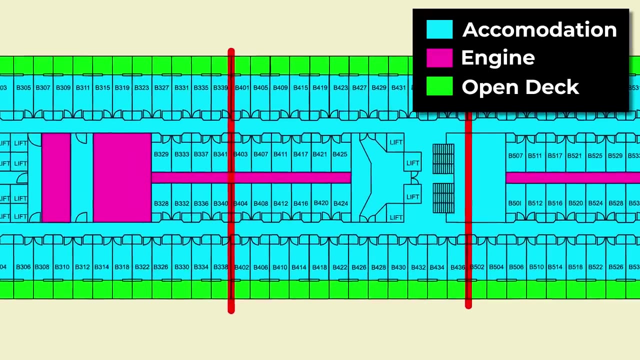 The ship was finally released to shore, where they eventually docked around 0945.. So how did it even get to this? How did the fire spread so far and so fast? Well, the primary issue was that the fire was on the balconies, which, at the time, were. 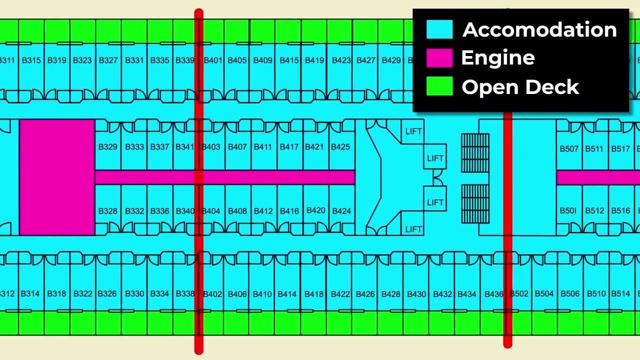 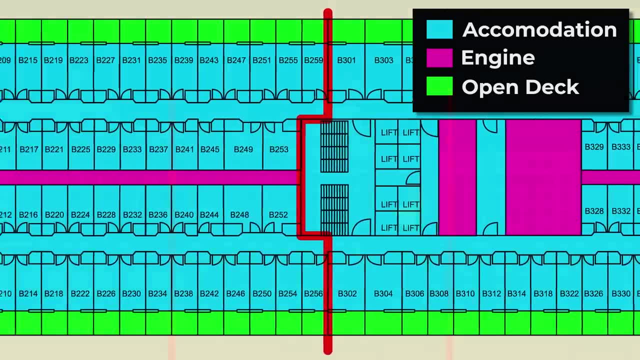 categorised as open deck spaces. This meant that they had different fire protection requirements from the cabins, such as fewer combustibility limits and less in the way of fire detection and suppression. It also gave the fire easy access to adjacent fire zones, allowing it to spread. 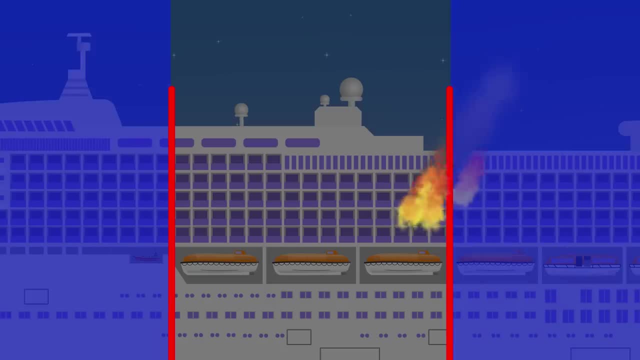 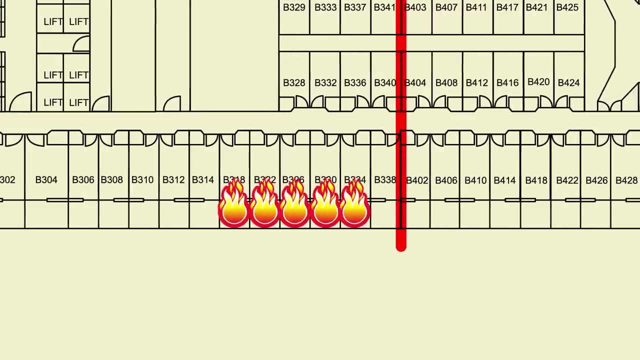 Ordinarily, you would expect a fire to remain contained horizontally within a fire zone, with boundary cooling above and below to stop it spreading vertically. In this case, however, the flames simply went around the zone boundaries, tearing along the side of the ship. 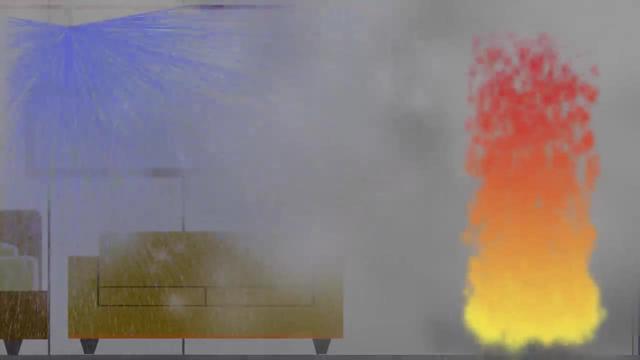 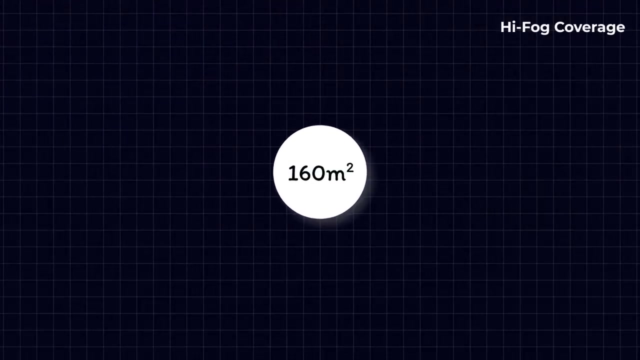 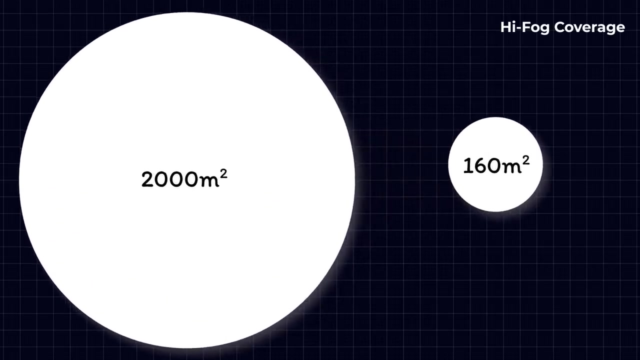 Fortunately, the high fog system did manage to keep it contained to the balconies, which was more luck than planning. The system had been designed to meet regulations which state that it must provide coverage for at least 160 square metres. On that night, it's estimated that instead, it managed to protect in excess of 2,000 square.